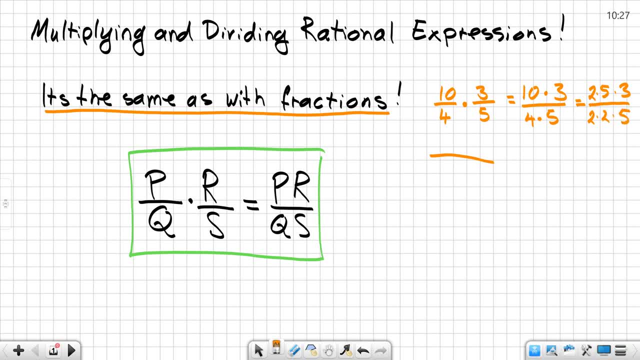 And I see that 4 can also be factored, Because what is happening right now is that I see that there are common factors in the numerator and denominator. Common factors cancel out, And I am just collecting the rest. So what is left here? 3 over 2.. 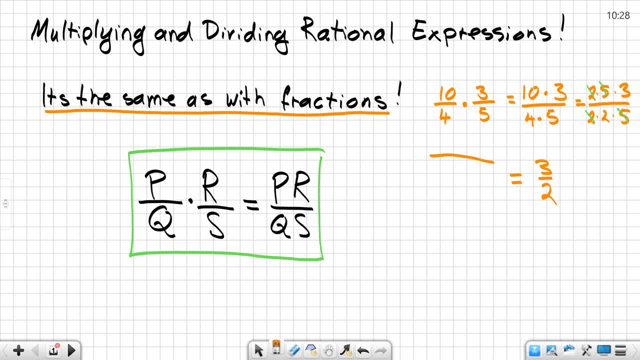 This is the exact same thing that we are doing with rational expressions. If I have a rational expression- p over q- and I multiply it with r over s- then what I'm doing, I multiply this straight across. Of course, I will always simplify before I write down my answer. 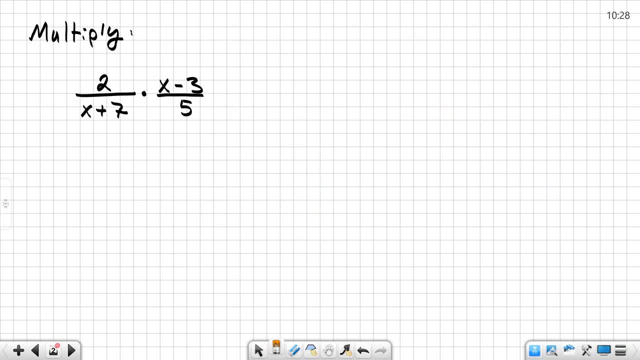 or multiply this actually out. So let's do an example. We are supposed to multiply 2 divided by x plus 7 with x minus 3 divided by 4.. So what I'm going to do? Alright, this is multiplication. Now be careful. 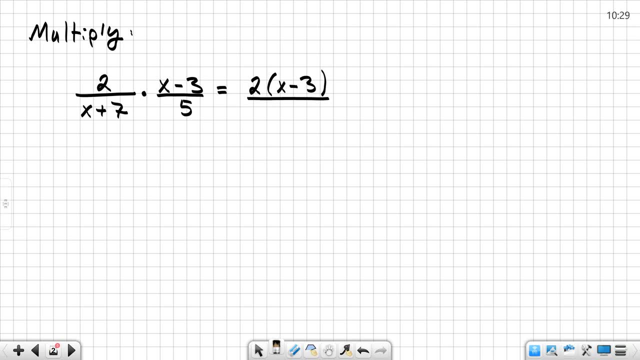 I have to put parentheses around x minus 3, because I have to multiply it with all of that right thing, And I will have to place parentheses around the x plus 7.. So now I'm looking at this and I see that there is nothing really. 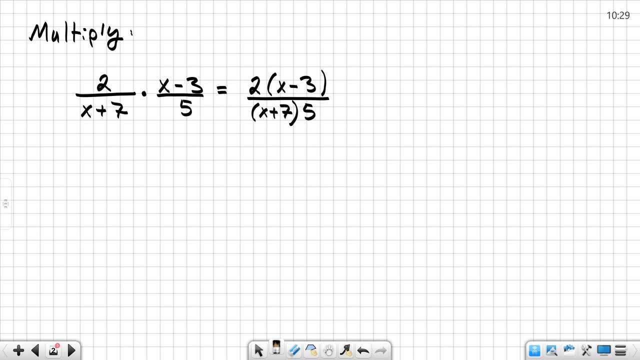 that I can factor any further. x plus 3, and x minus 3 is what we called prime, And then I can just multiply this out. In the more complicated example we leave it in the factored form, But because this is fairly simple to just multiply out, 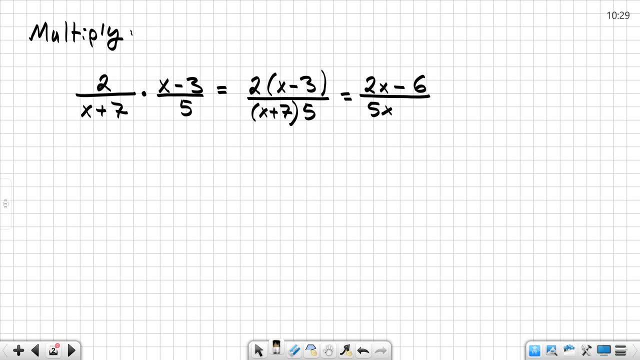 we are just going to go ahead and do this. So 5 times x is 5x, 5 times 7 is 35. And that is it. So let's do another example: x plus 4 over x minus 7, multiplied with 3x minus 21. 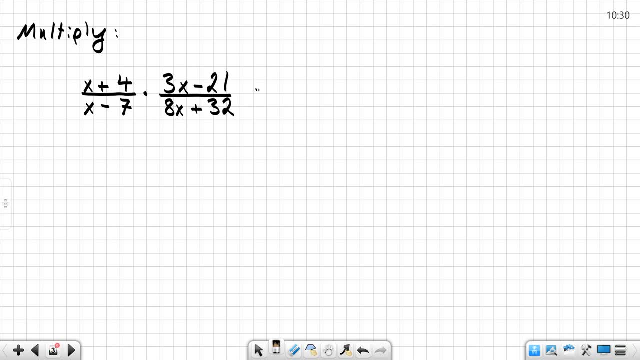 divided by 8x plus 32.. Again, factoring, factoring, factoring. If there is anything you can factor, then you can factor it. So let's first write it down as before. So what I'm doing, I really multiply straight across. 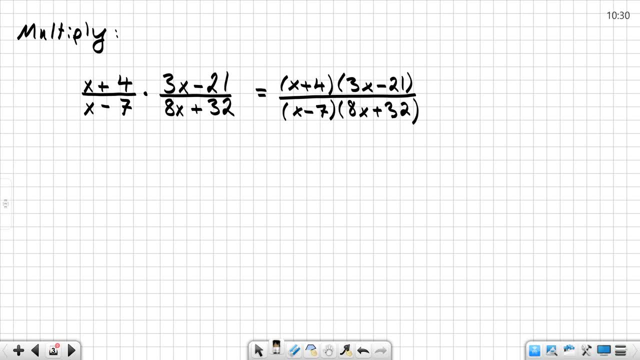 But instead of multiplying this out right now, which would be way too complicated, I am looking at my second factor up here: 3x plus 21.. This factor right here can be factored. There is a common factor of 3x. 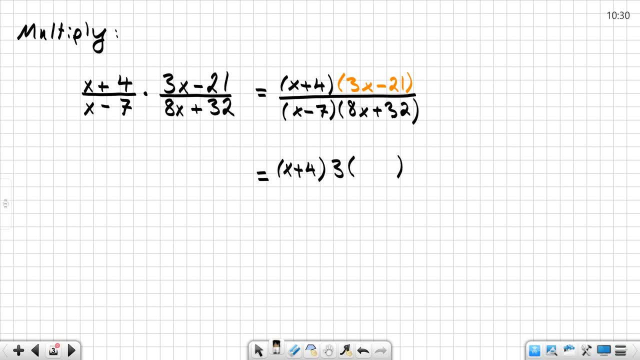 There is a common factor of 3, that is, in both terms. The GCF was 3.. I take it out of the 3x, I'm left with the x And I take it out of the negative 21.. I'm left with negative 7.. 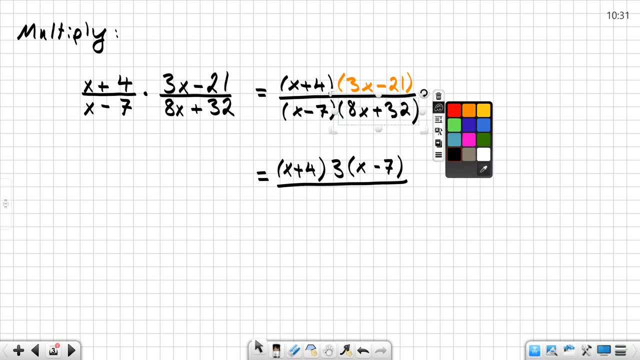 I'm going to do the same thing with this one right here. This also can be factored 8x plus 32.. There is a common factor of 8.. I'm writing in both terms And if I take out the 8 out of 8x. 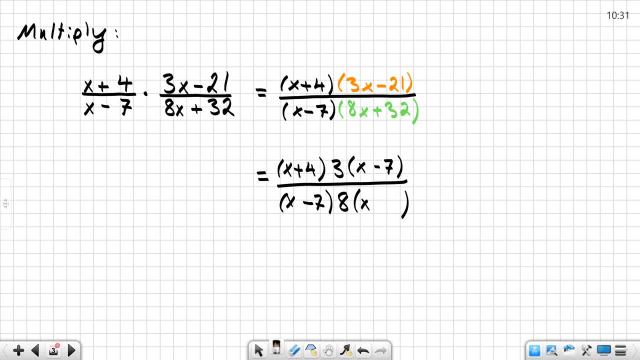 I'm left with an x- Let's make this a little bit nicer- And 8 divided into 32, or, in other words, if I take it out as a factor of 32, I'm left with 4.. All right, 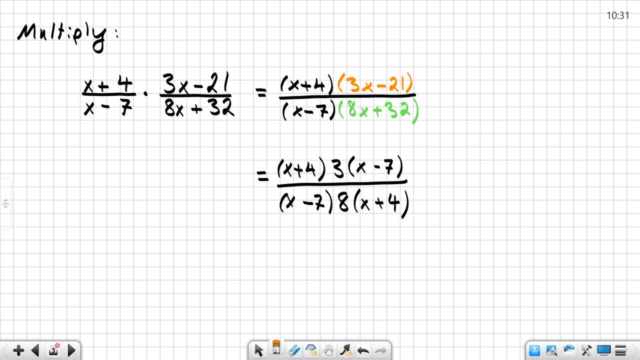 Now I step a little bit back or I look at my paper. if I'm working this out, Then I see right now that there was a factor of x plus 4 in the top and the bottom And there is a factor of x minus 7. 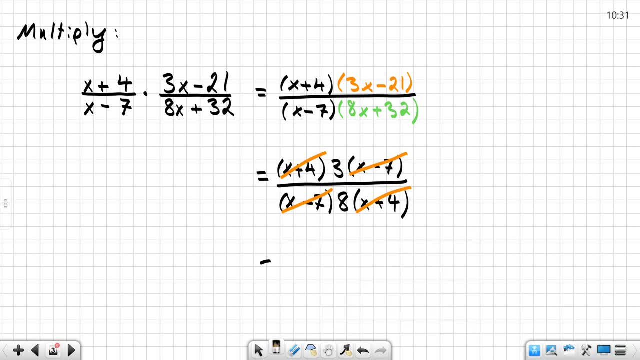 in both numerator and denominator, And that means now all that is left is 3 divided by 8.. Let's do another one: x minus 5 divided by x minus 2.. We want to multiply this with x squared minus 4,. 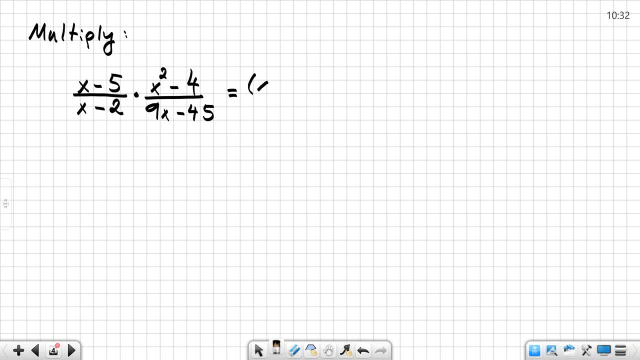 divided by 9x plus 45.. So again, I am rewriting everything. But instead of writing now times x squared minus 4, I will immediately take this right here and I will factor this: x squared minus 4, this can be factored. 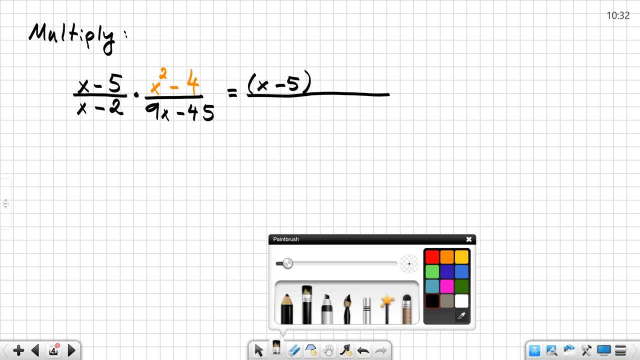 This is, you see, how all of our rules for factorizations are coming back in this section. x plus 2. Plus 2 times x minus 2. This was the difference of two squares, And 9x minus 45 can also be factored. 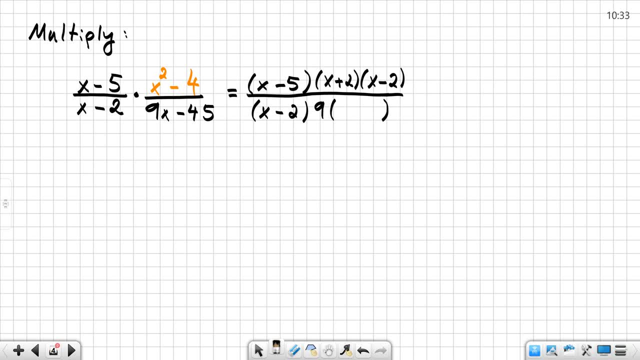 There is a factor of 9 in 9x, leaving an x, And there is a factor of 9 in negative 45,, leaving a negative 5.. Now I'm going to look. This is now the fun part. This is the best part of these problems. 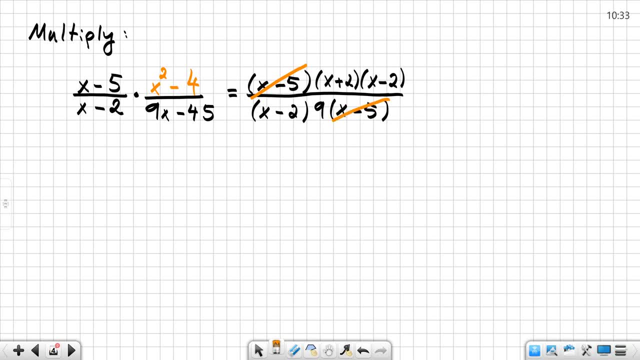 I look There is a factor of x minus 5.. There is also a factor of x minus 2. And I just have to collect the rest. I'm just writing down the answer: x plus 2 is the only factor there is. 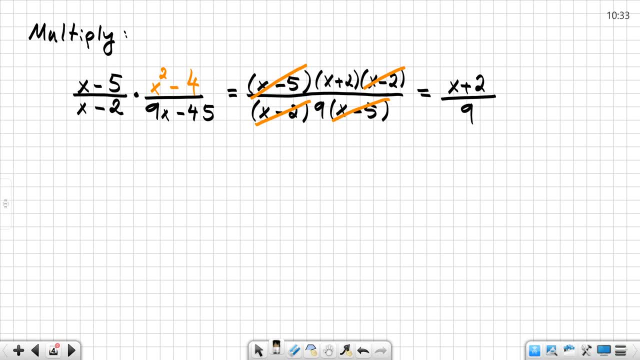 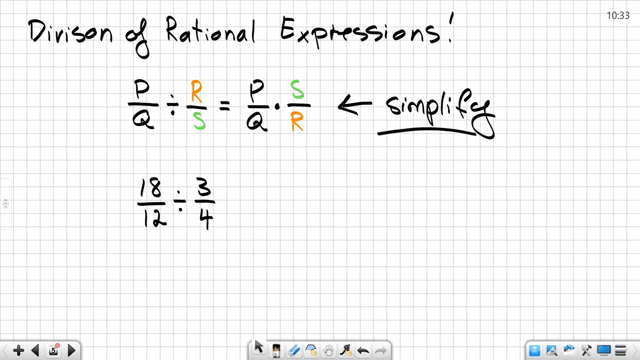 That means I can leave the parentheses of. If you would put parentheses around this, this doesn't make it wrong, This is just not necessary. So we leave those parentheses off. All right, Let's do something different. Division- If we are dividing rational expressions, 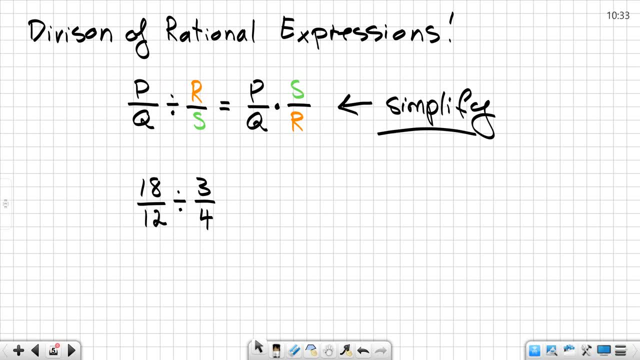 then with algebra we always have these letters. So if we write it down as a rule- p over q- And I'm dividing this now by r over s, What I'm doing is I just flip the second one around and I get s over r. 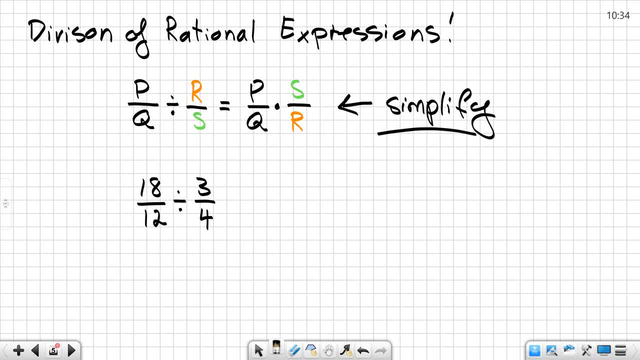 You might have learned: copy, dot, flip or copy, whatever all of these little funny sentences were that helps you to remind that you have to take the reciprocal of the second one. This one is the one that we are just flipping around And we turn it into multiplication. 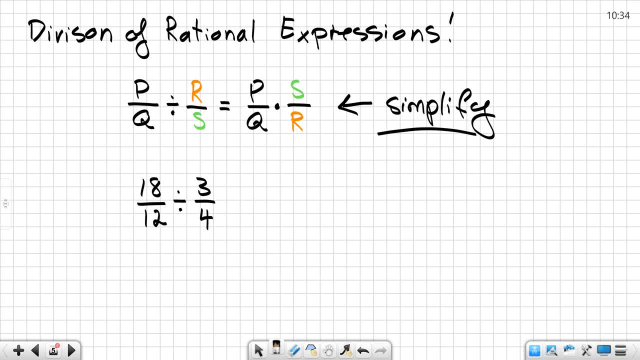 Copy dot flip has some sort of a ring to it. Let's do an example right here with numbers, All right, So 18 divided by 12, divided by 3, divided by 4.. Remember, this is also nothing else really, but division. 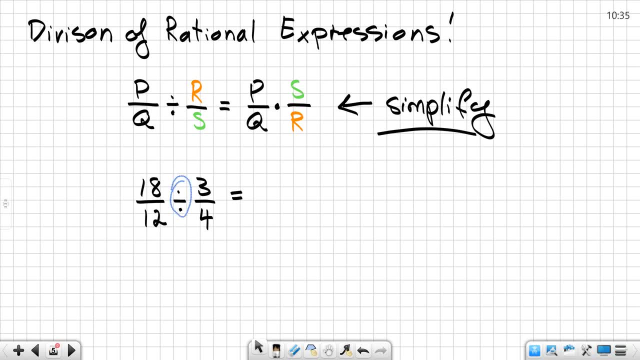 So this dash right here, this fraction and this division sign really is the same thing. We will see this later. But what I'm doing now in this problem: I copy down the first fraction, I turn the division into multiplication and I flip the second fraction around. 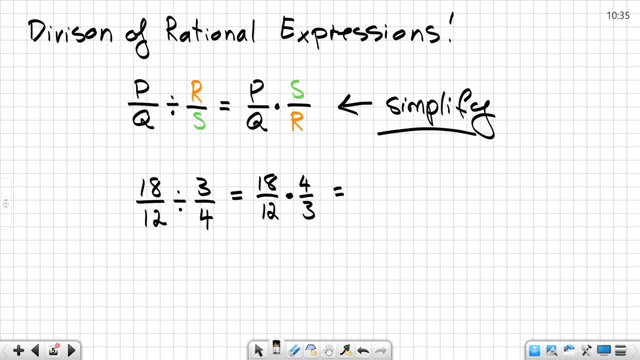 I take the reciprocal, Now I am multiplying straight across. So, in other words, now it's exactly like we did before, And of course, you would not multiply 18 and 4.. What I would do now I am breaking this down into as small pieces as I can. 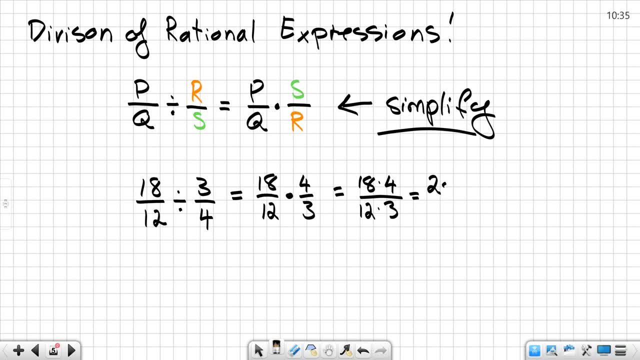 18 is the same thing as 2 times 9.. And 9 is the same thing as 2 times 3.. 2 times 3 times 3 is the same thing as 18.. 4 is the same thing as 2 times 2.. 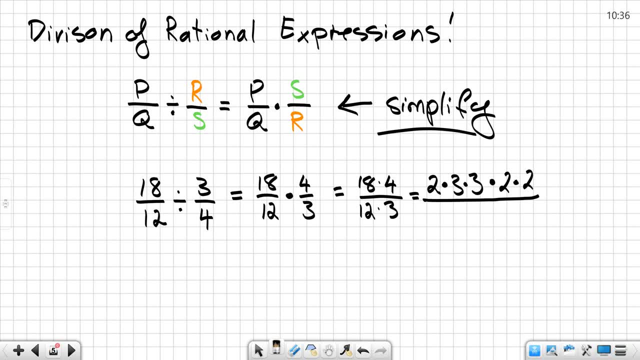 What I just did here is called the prime factorization of a number. 12 is 3 times 4.. 3 times 4. And 4 really is just 2 times 2. Times 3.. So now I see all factors. 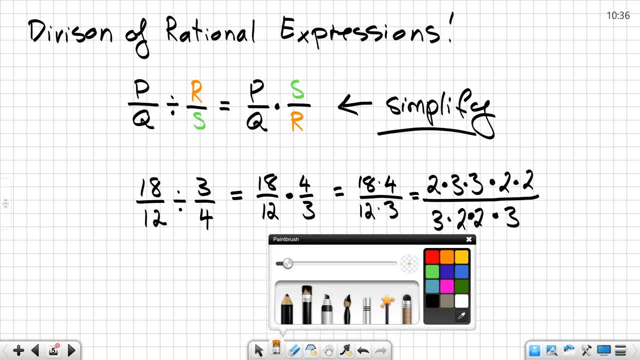 Oh, there are a lot of factors, And what I do right now I just pair them up on the top and the bottom. There is a factor of 2.. There is a factor of 3.. There is a factor of 3.. 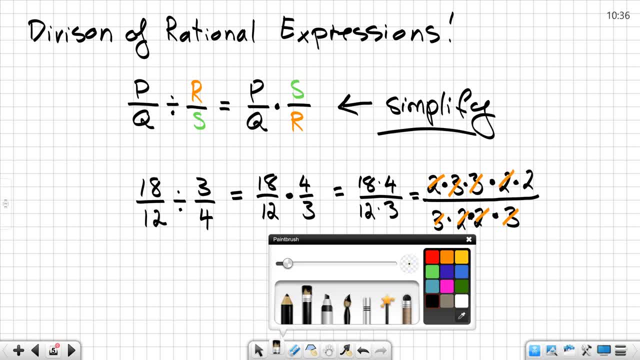 And there is a factor of 2.. Oops, All that is left is 2.. Well, what is left in the bottom? Don't say nothing. There is always a 1.. I do not need to write this: 1.. So, in other words, 18 divided by 12. 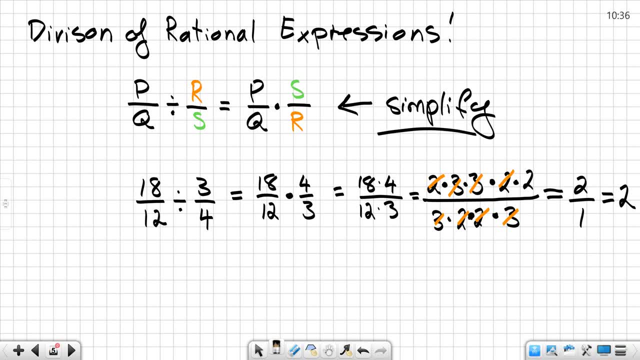 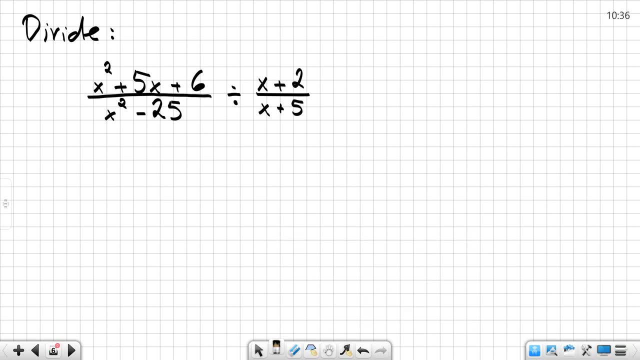 multiplied, divided by 3 over 4, is nothing else but 2.. Let's do this with rational expressions. So if I have the following problem right here and I am supposed to divide, then what I am going to do, I am going to rewrite this problem. 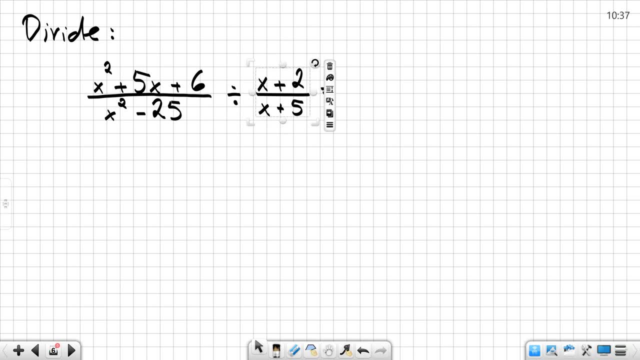 and I am going to take this one and write it upside down, In other words. well, I cannot really do this with my little tool right here. I am going to flip it upside down, so to speak, But so that I don't write too much. 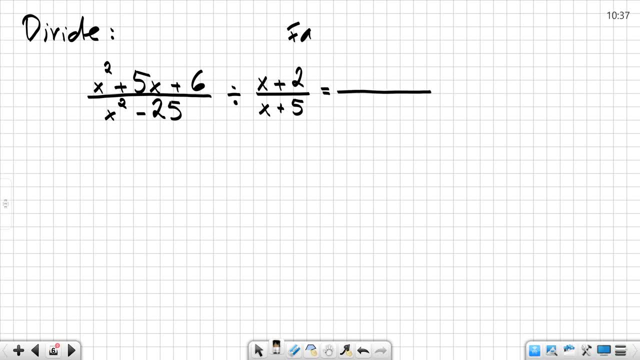 I will immediately factor if I see something can be factored: x squared plus 5x plus 6, this is the same thing as x plus 2 times x plus 3.. 2 times 3 is 6.. 2 plus 3 is 5.. 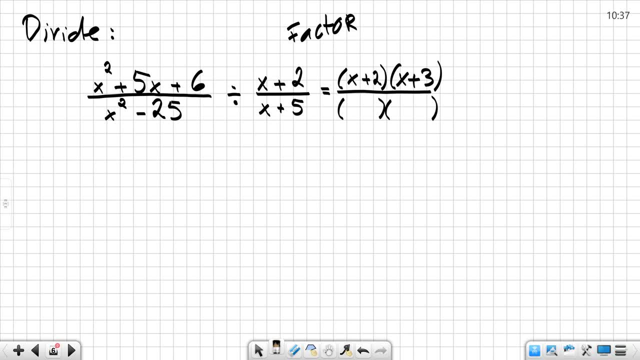 On the bottom, what I see is the difference of two squares x plus 5 times x minus 5.. Now I turn this division into multiplication and I am flipping this second fraction upside down. And now what I can do now? now I multiply straight across. 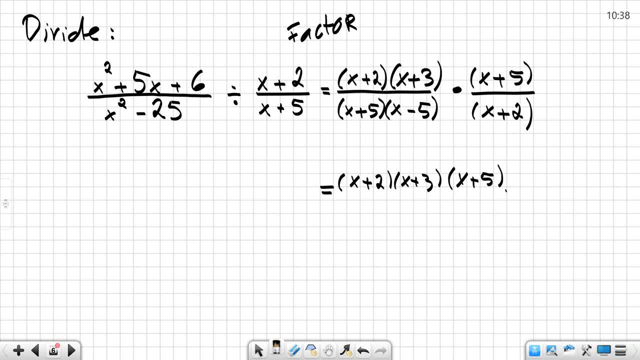 Well, I could already now cancel out, but let me write it down exactly like I did before: Times x plus 2.. And you see, the really the only, the only really complicated thing is the factoring, Because now what I am doing, 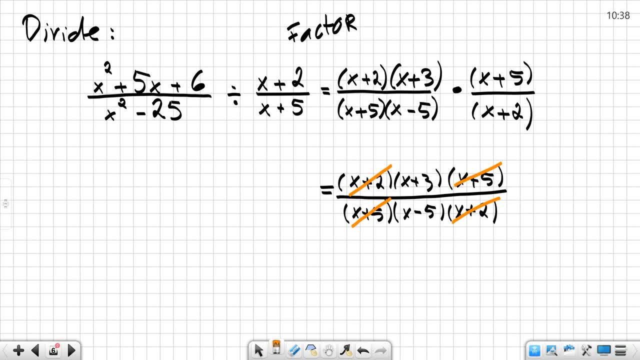 I am searching for common factors. I cancel out as many factors as I see that are the same in the top and the bottom, And then I am just going to collect the rest. x plus 3 divided by x minus 5 is all that is left.